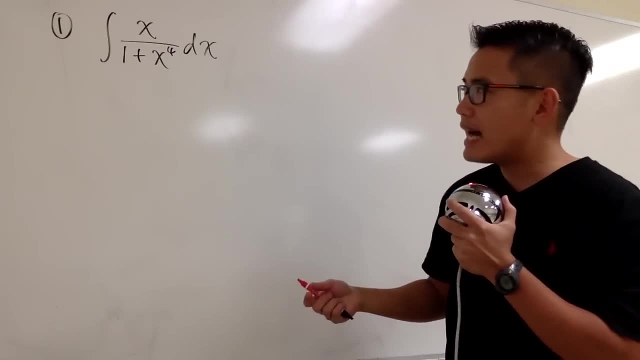 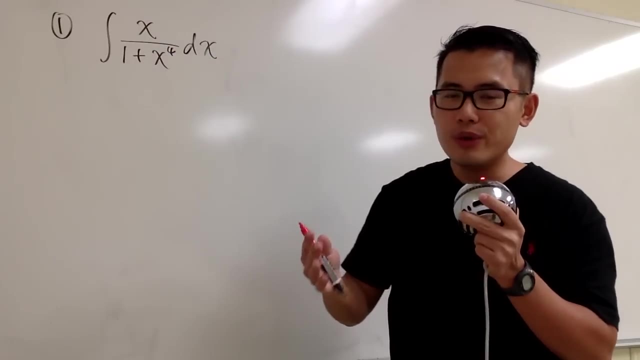 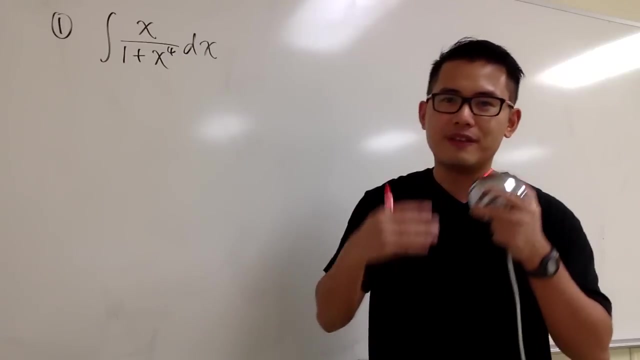 right, So u should be what? So that we can cancel this? x to the first power? Well, this is x to the first power. i want to let u equals to something with x to the second power, because once i differentiate that, i get something x to the first power, isn't it okay? i want to. 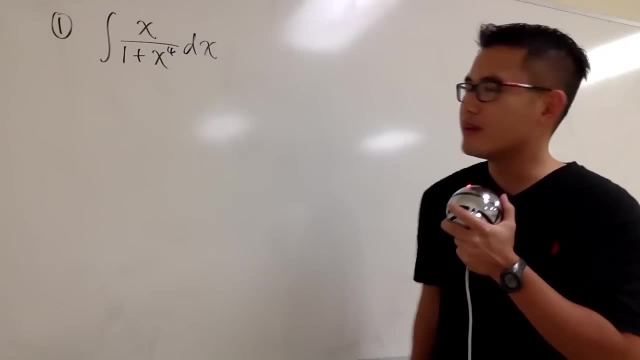 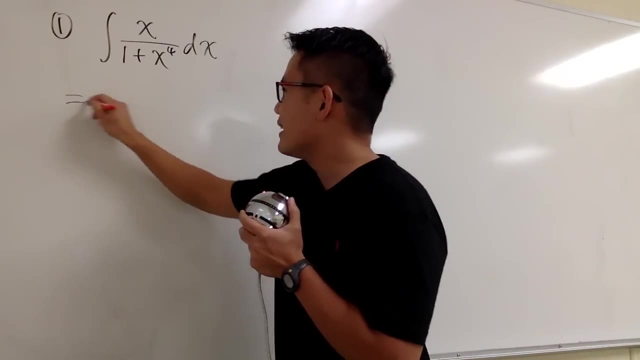 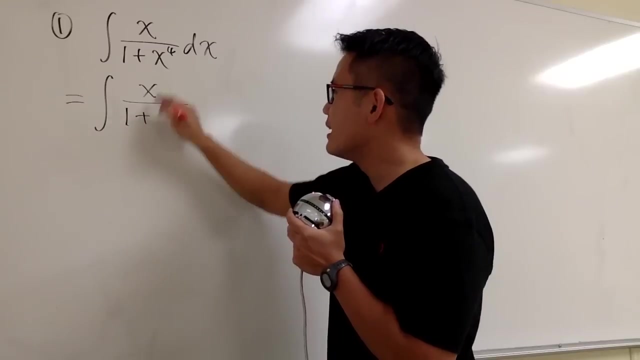 produce x to the second power somewhere in this integral and the place it's going to be right here. let me show you. okay, okay, i'm so excited, all right, so this is going to be the integral on the top, i'm just going to let it to be x, and on the bottom we have one plus instead of this, x to the fourth. 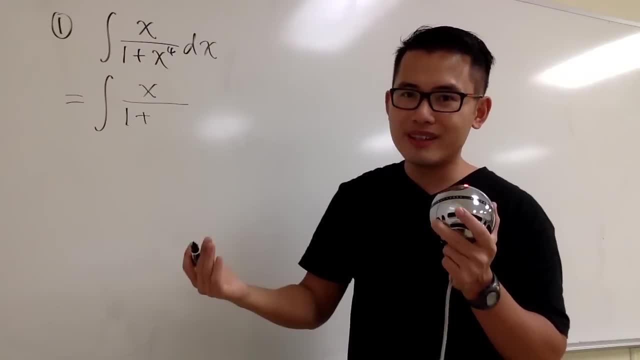 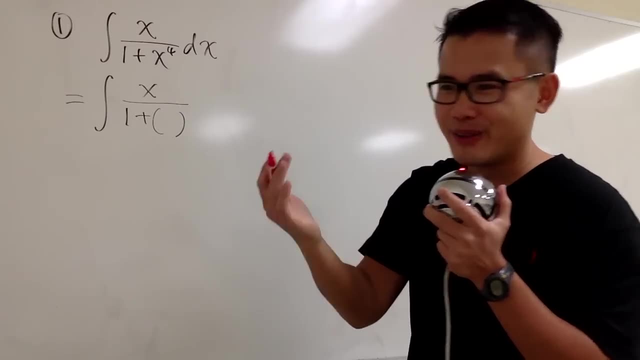 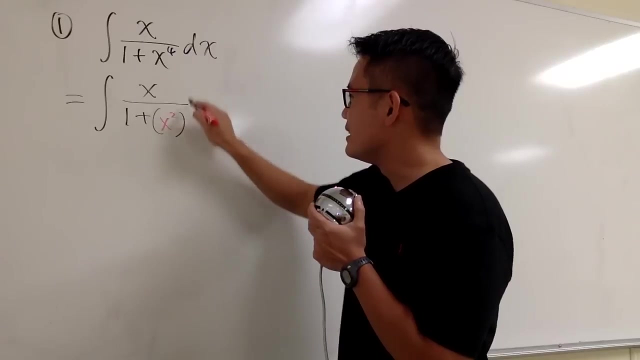 power. let's look at this as x- square and then square. how's that? so i'm going to open the parentheses and you see, i'm going to just switch the marker like this. this is so cool. huh, inside here i will put down x to the second power and then this to the second power, so that this is: 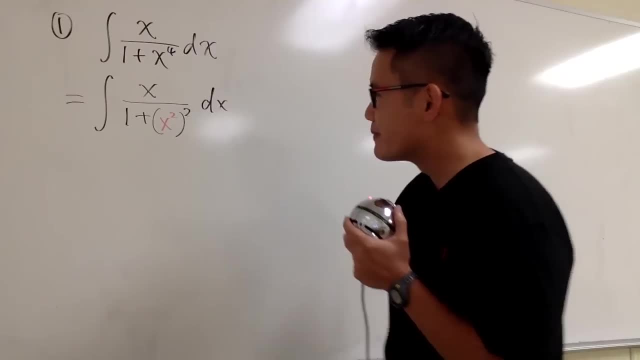 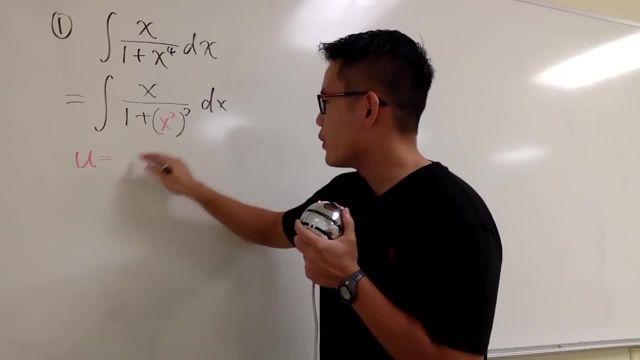 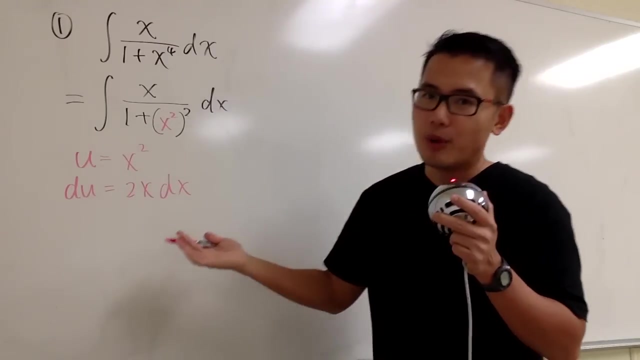 the fourth power, isn't it? this is just so cool. and now, what? well as our strategies earlier, i'm going to let u equals to x squared right here, so that when i differentiate it, i get: du is equal to 2x dx. same old business. let's divide 2x on both. 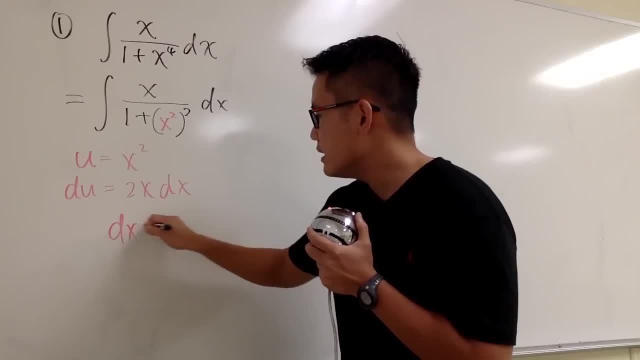 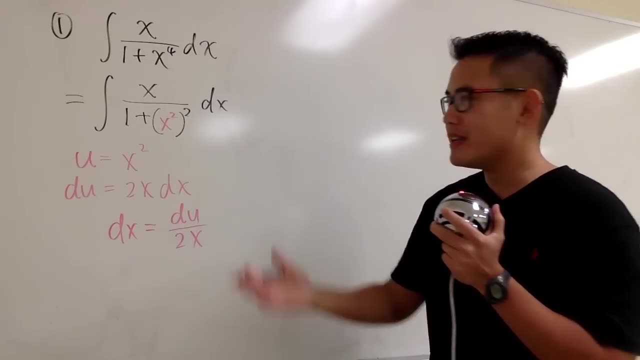 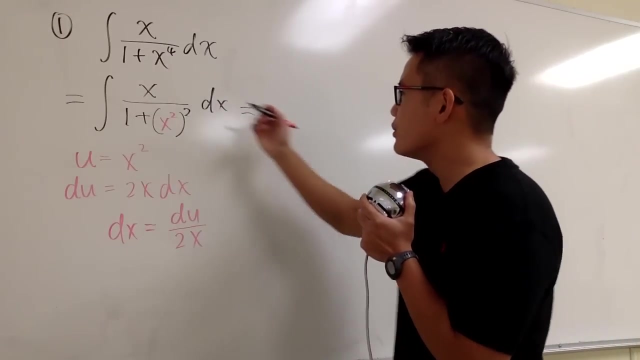 sides so we can isolate the dx. so we get dx equals to du over 2x. and now we can take this integral from the x world to the u world and now we will see this is going to be the integral x on the top, over one plus. 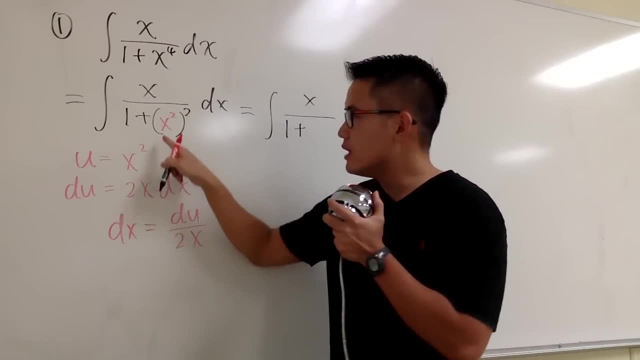 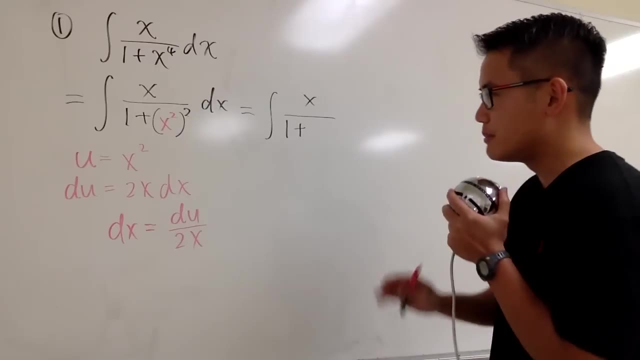 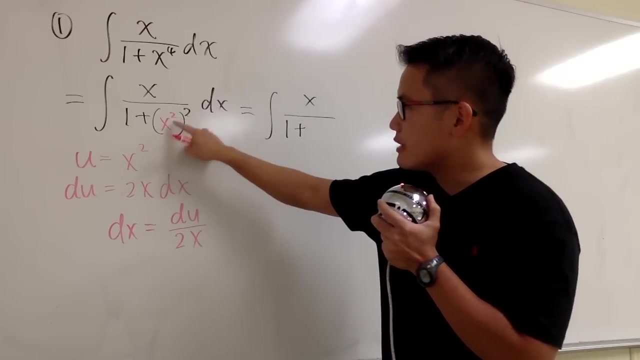 and notice that i only let u equals to x squared, because inside here we only have x squared. that's the inside function, right? i cannot say one plus x squared, okay, so that's very different. therefore, we still have the one plus right here and then the inside u. this is x squared, actually x squared, that's. 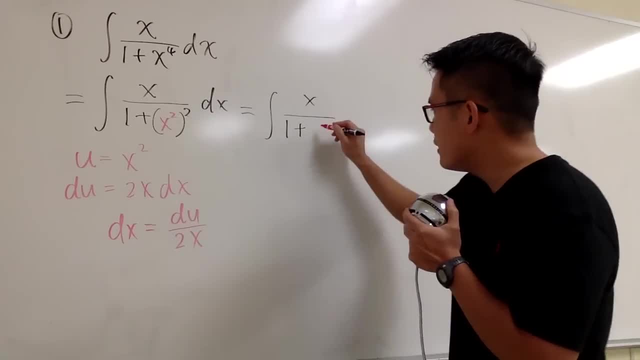 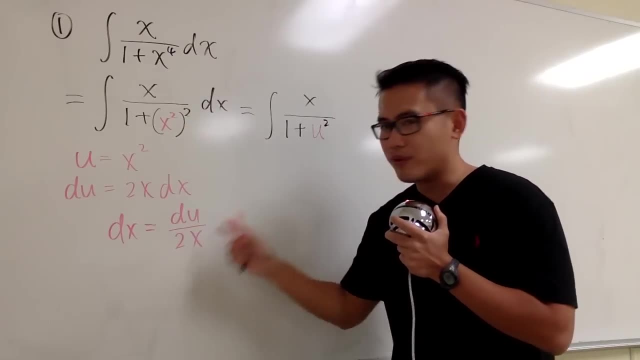 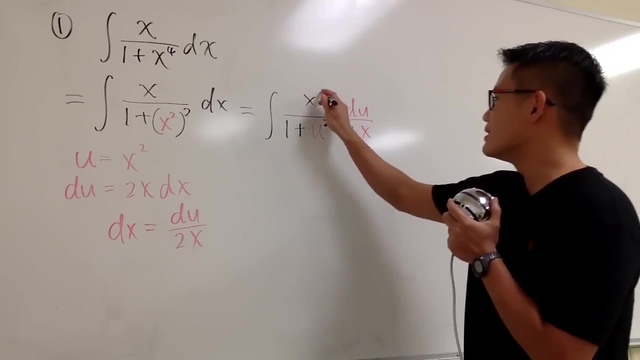 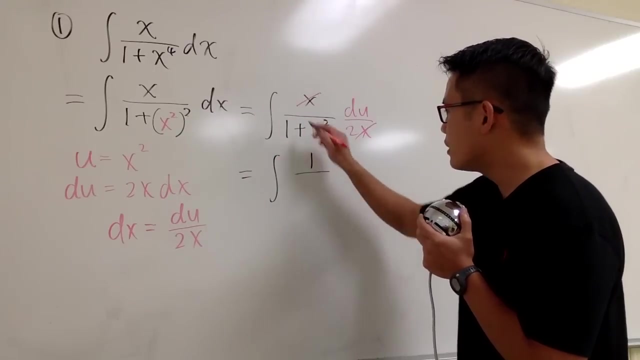 the u. okay, i'm going to change that. it was x squared and now it's going to be the u, and then we still have that to the second power. and then for this, dx is du over 2x, so let's put that down: du over 2x, very nice, so that we see this x and x cancel each other, huh. and then we are just going to be integrating one over one plus u squared du, and now let's see the u, and then we still have that to the second power. and then for this dx is du over 2x, so let's put that down: du over 2x, very nice, so that we see this x and x cancel each other, huh. and then we are just going to be integrating one over one plus u squared du, and now let's see the u, and then we still have that to the second power. and then for this dx is du over 2x, so let's put that down: du over 2x, very nice, so that we see this x and x cancel each other, huh. and then we are just going to be integrating one over one plus u squared du, and then we are just 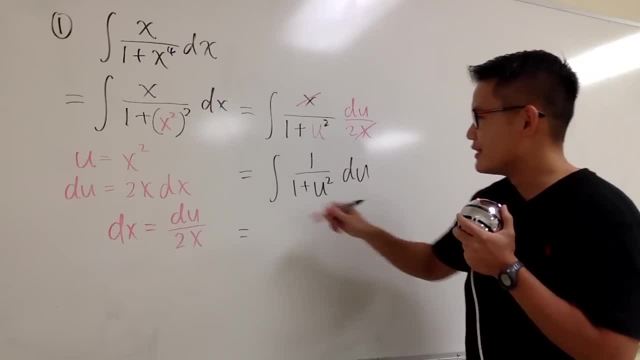 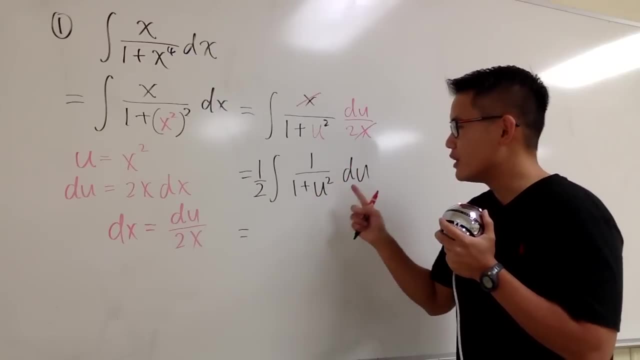 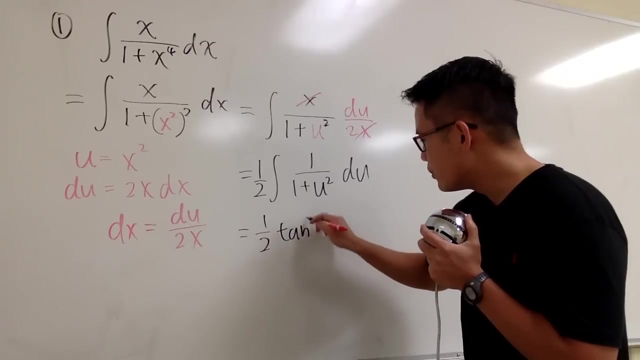 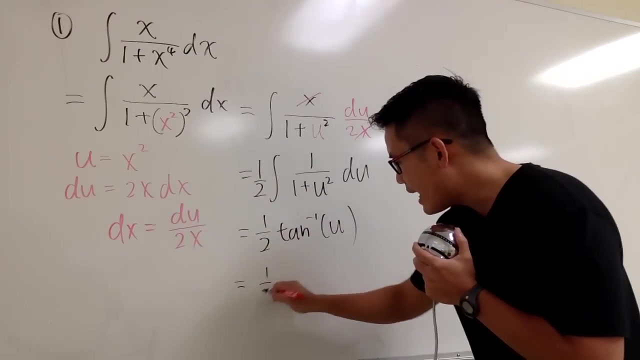 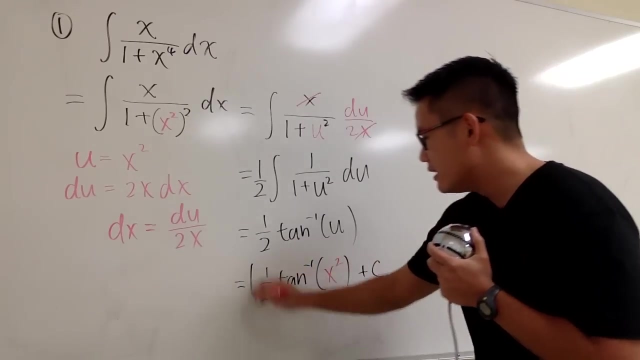 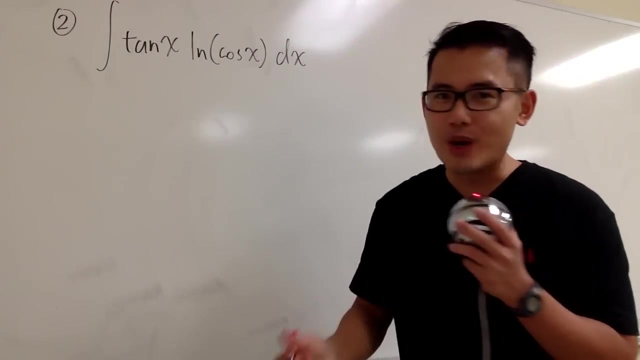 going to be integrating one over one plus u squared du, and then we are just going to be integrating one over one plus u squared du, and then we are just, we are done. so put plus c this right here. that's it really cool, isn't it okay for the second one? 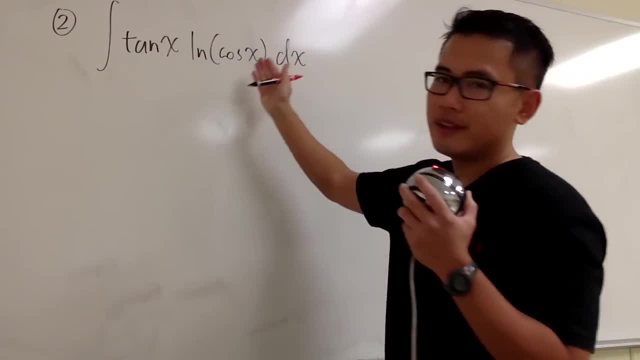 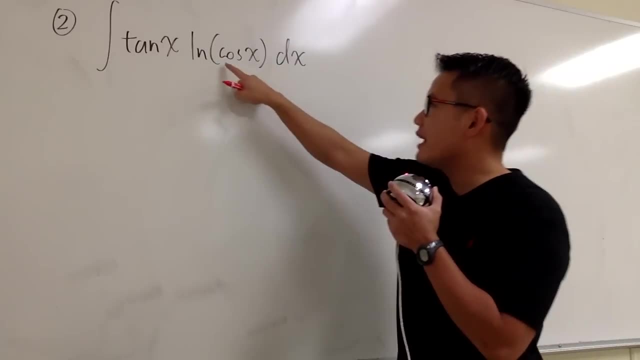 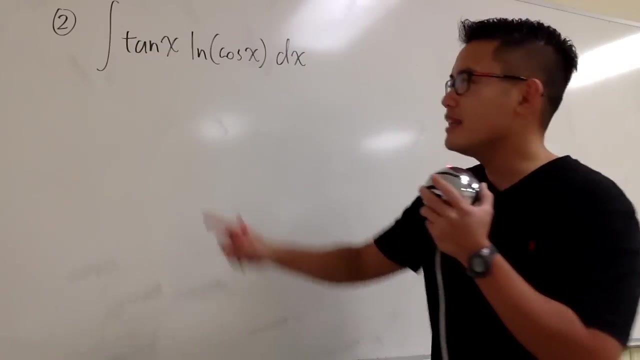 we have the integral of tangent x times ln of cosine x. as usual, I like to tell you guys: okay, maybe we let. u is equal to the inside function. however, in this case, if u is equal to cosine x, the derivative of cosine x is negative sine x, and here we don't have a sine x. this is: 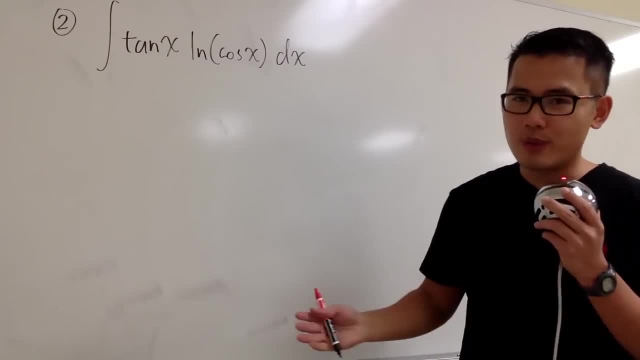 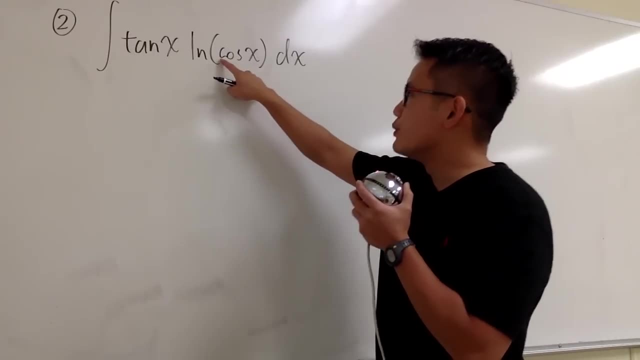 what tangent x, so they don't cancel each other out right away. right, maybe it will work, maybe not, I don't know. but here is the secret: instead of letting u equals to cosine x, I'm going to let 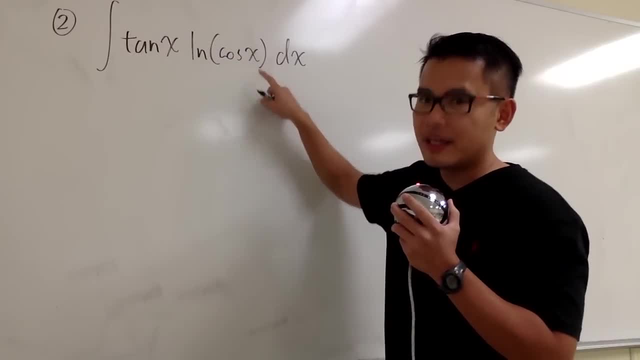 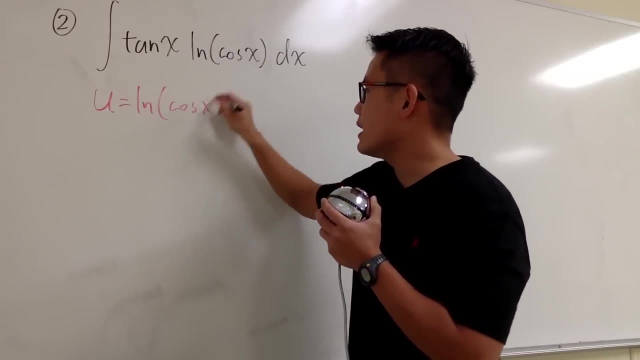 u equals to ln of cosine x, and let me show you why I chose to do that. so u equals to ln of cosine x and I'm going to differentiate this for you guys. you will see du is equal to. and now remember how. 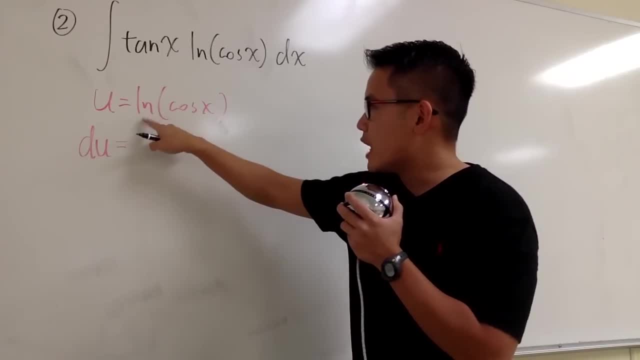 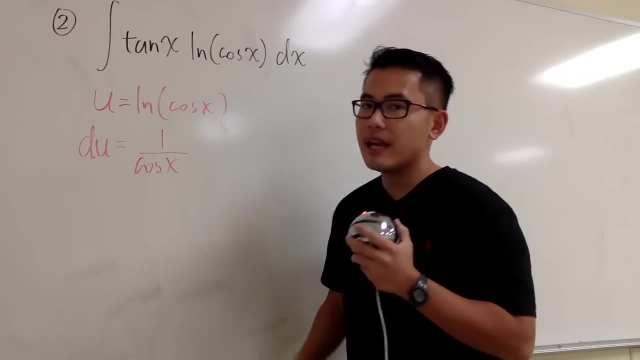 to differentiate. differentiate with the ln function derivative of ln of something is going to be 1 over the inside right and the inside stays the same for now. so we have cosine x. but don't forget, the chain rule says we are going to look at the inside and then you know, look for the derivative of this. 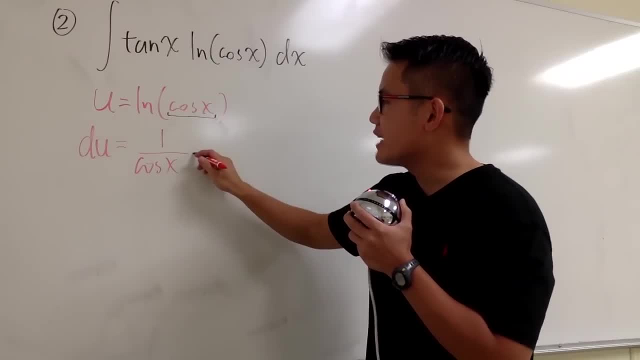 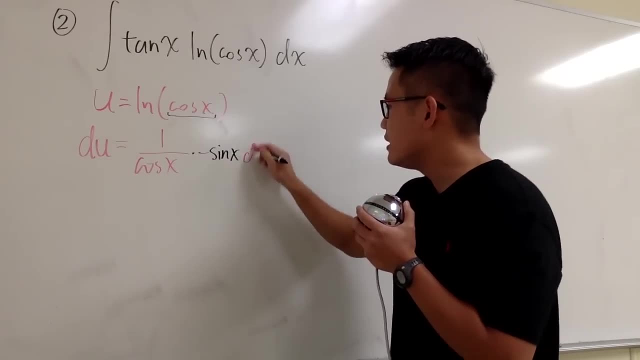 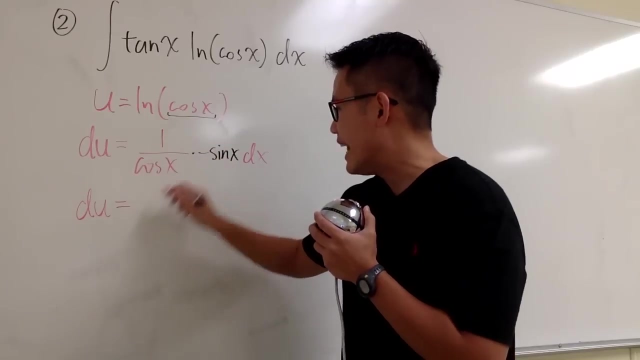 the derivative of the inside derivative of cosine x is negative sine. so we multiply by this, by negative sine x. okay, the chain rule, and we still have the dx. and now I'm going to just rewrite this again: this is: du equals to negative. we have sine x over cosine x. 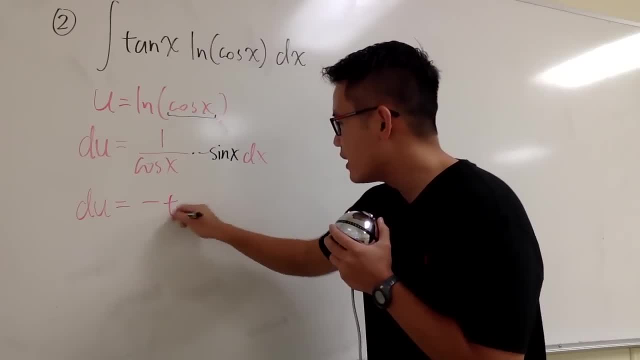 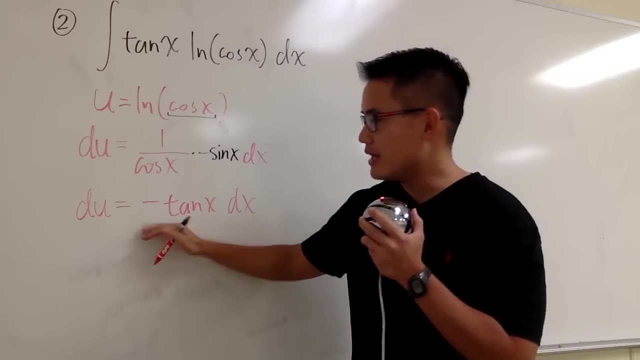 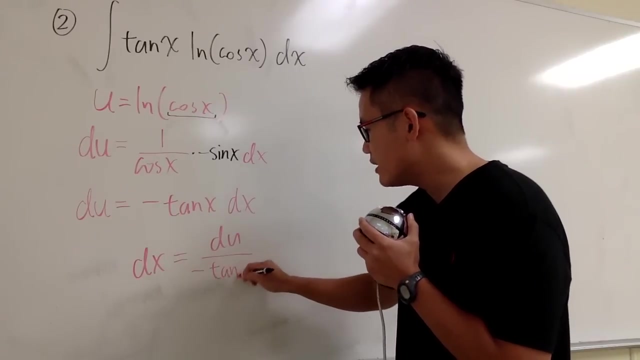 so that's what that's tangent x. so this is negative tangent x, dx, and you see, I'm going to divide both by negative tangent x so I can isolate the dx. dx will be du over negative tangent x, and you see now, 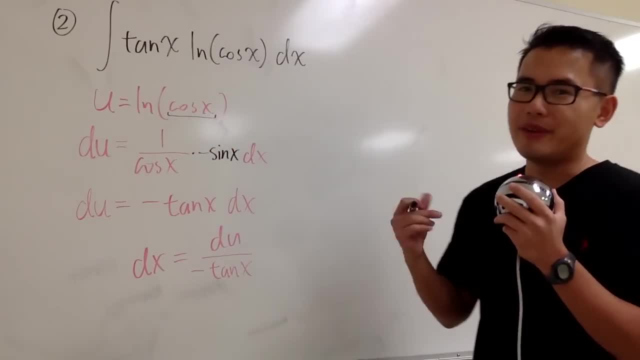 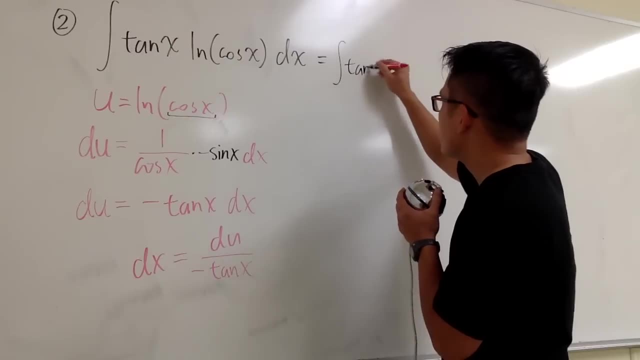 This tangent x and that tangent x will cancel each other out. Very nice, huh? All right, take this integral from the x world to the u world. This is going to be the integral tangent x times this part, the whole, this right here. 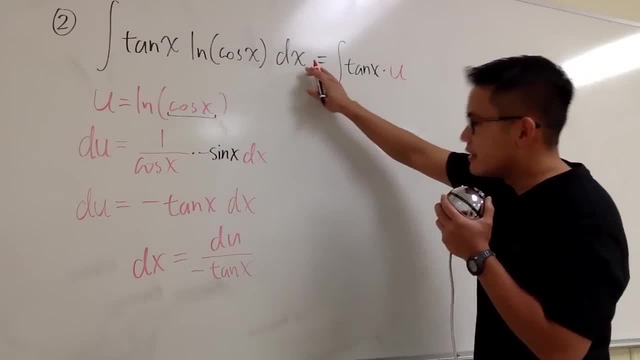 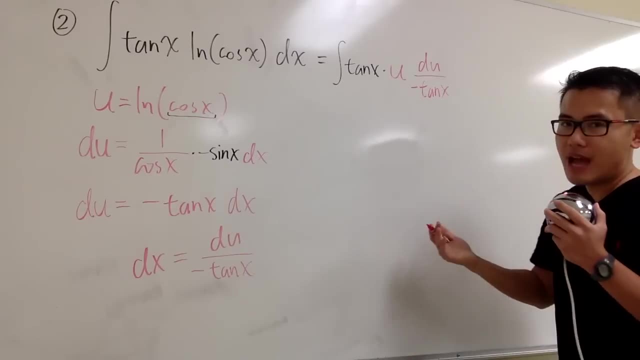 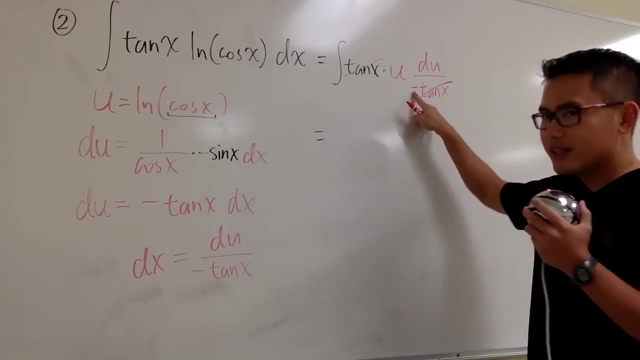 It's the u, so I will multiply by u And then the dx. is that du over negative tangent x, And now tangent x, tangent x. cancel each other out And we will have what? Don't forget? the negative. 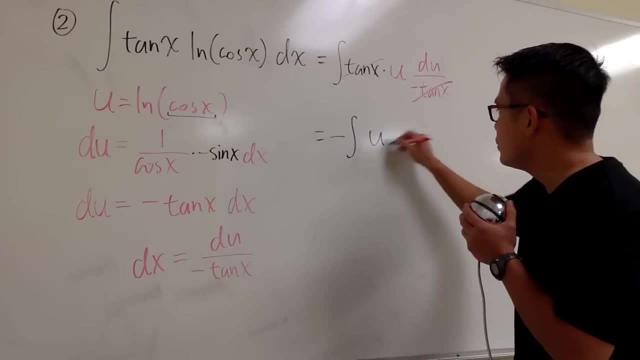 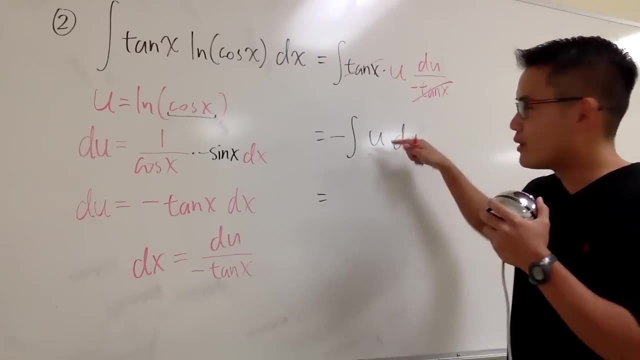 Bring the negative to the front. Negative integral u du. And how do we integrate u in the? u world? Well, this is going to be your other power: 1 plus 1 is 2.. And then divide by 2,, which is the same as multiply by 1 half. 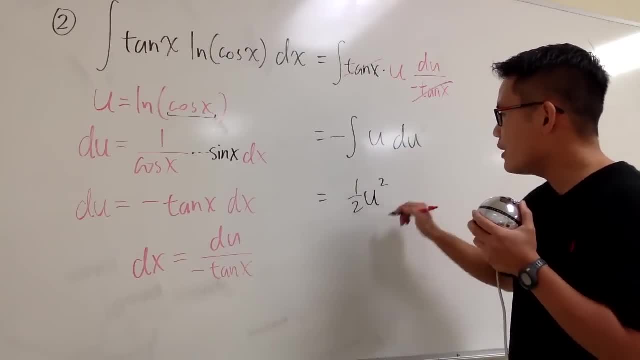 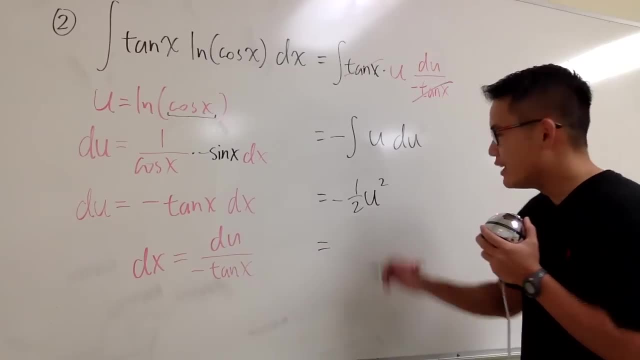 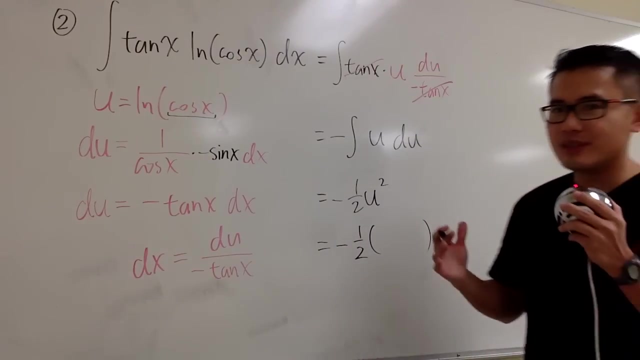 Anyways, this is going to give us 1 half u squared And we bring down Negative. Okay, we are done. At the end. I'm going to rewrite this: nicely, We have the negative 1 half right here, And then for the? u, let me open a parenthesis to make everything look clear. 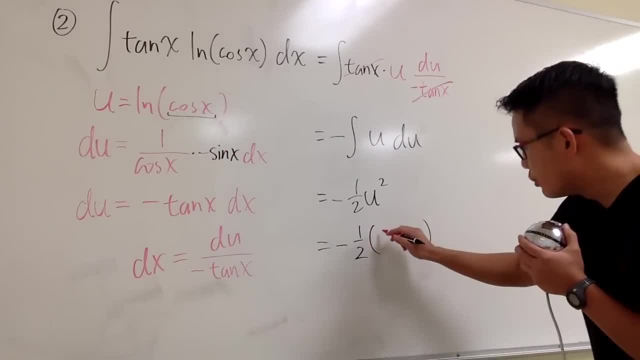 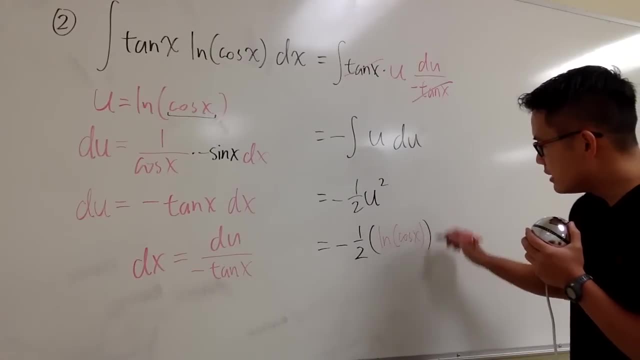 Inside here for the u, which is ln of cosine x. Let's put that down here: ln cosine x. And then we are going to raise this to the second power And we are done. So put a plus c, This right here. 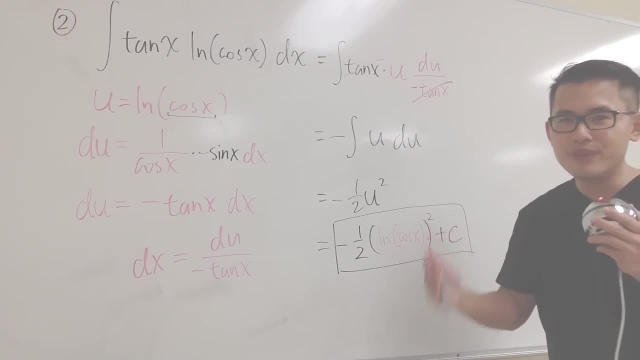 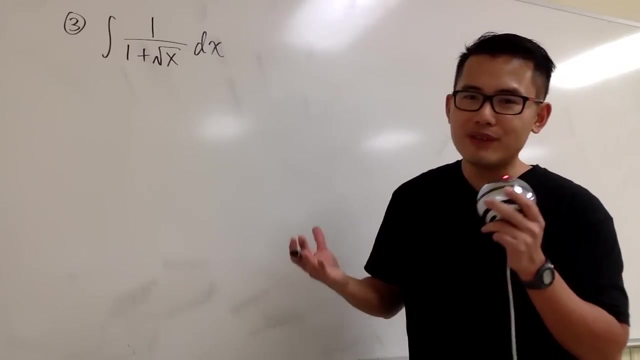 Is it Okay? And one more example for you guys. Okay, for this one, we have the integral of 1 over 1 plus square root of x. We don't have a lot to work with, isn't it? Because it seems like our only choice for the u is the denominator. 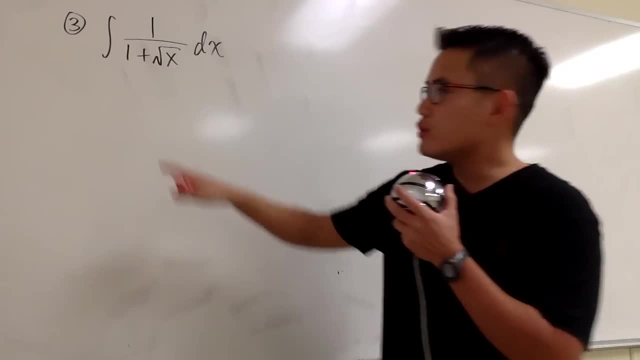 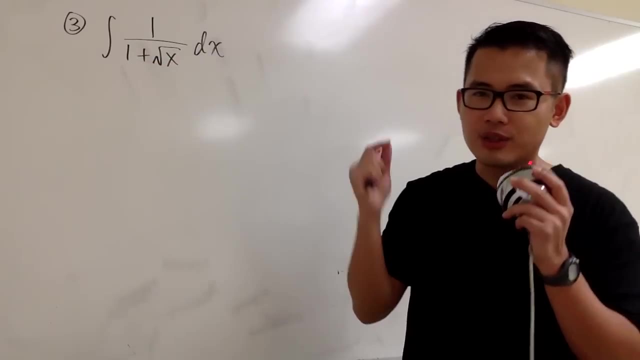 1 plus square root of x. And the reason that I want to attach the 1 plus right here is that when I differentiate the whole denominator, the 1 goes away anyways. So that's a good choice, And I'm not sure what will happen. 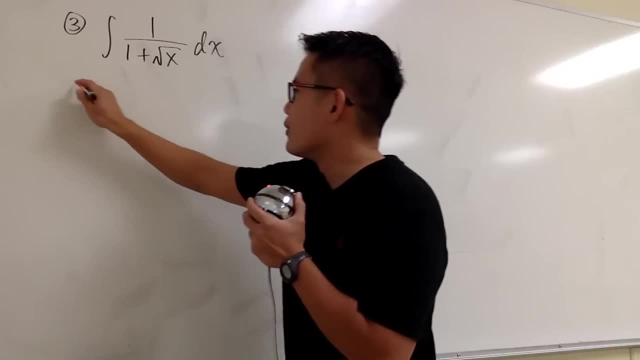 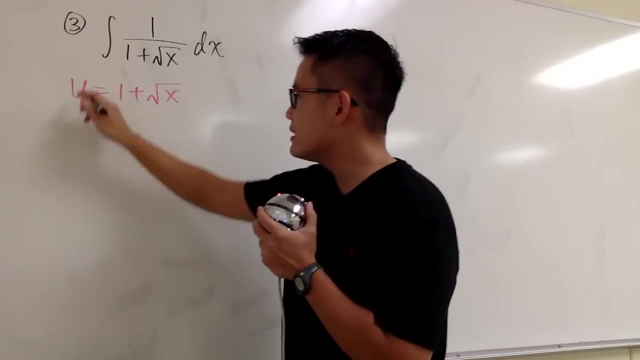 And let's just try our best to make things happen. Let's go u equals to the denominator 1 plus square root of x, And then I'm going to differentiate both sides So we get du equals to. this is 0.. Derivative of square root of x is what 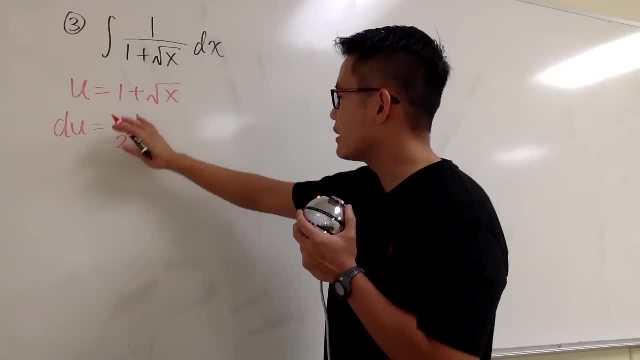 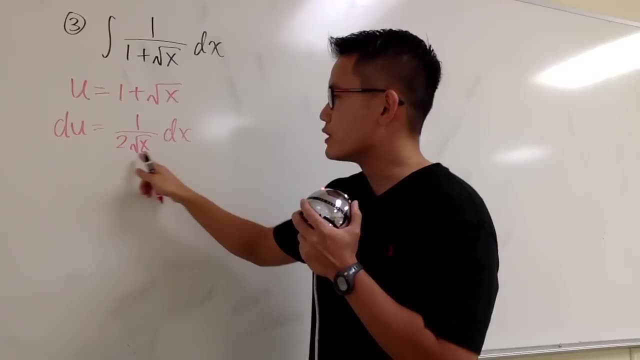 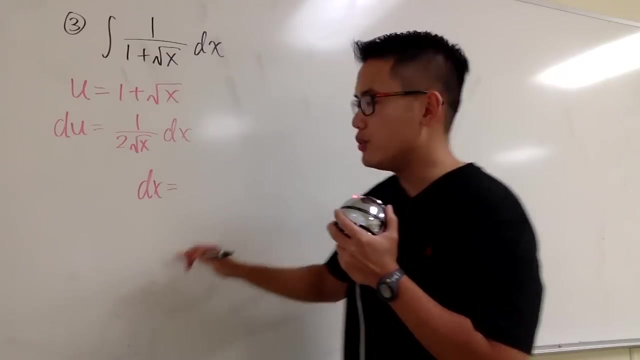 1 over 2 square root of x. And then we are done with the derivative part. So attach the x. This time we are going to multiply both sides by 2.. Square root of x, so that we can get dx, equals to 2 square root of x. du right. 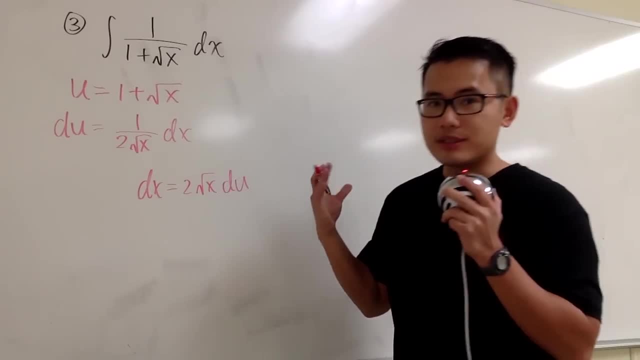 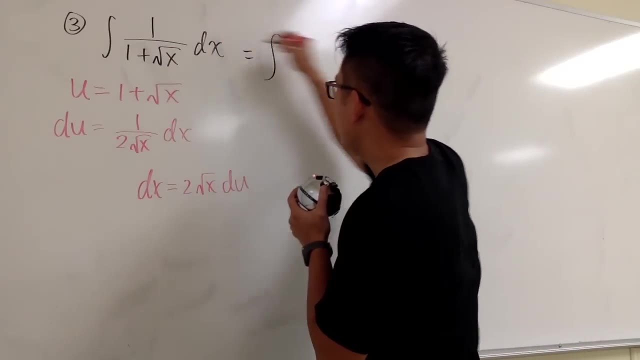 2, square root of x, du. And let's just take this into the? u world to see what we get. So this is going to be integral 1 on the top over the whole thing. right here is u. So I put down the u right here in the denominator. 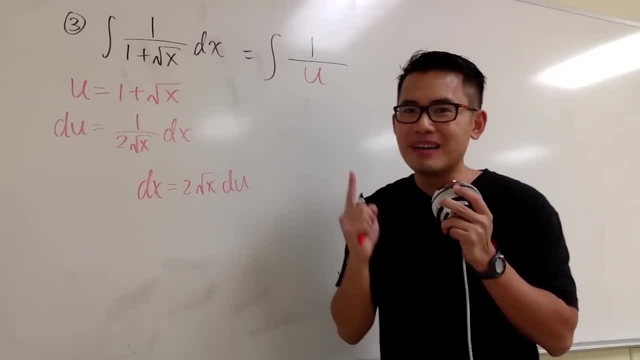 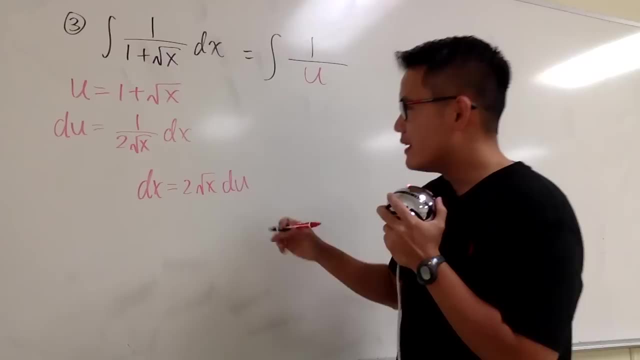 And then for the dx: we know it's this, But there's somebody that's not invited in the? u world. But there's somebody that's not invited in the? u world, Namely the square root of x. But the good thing right here is that, if you refer back to this equation here, 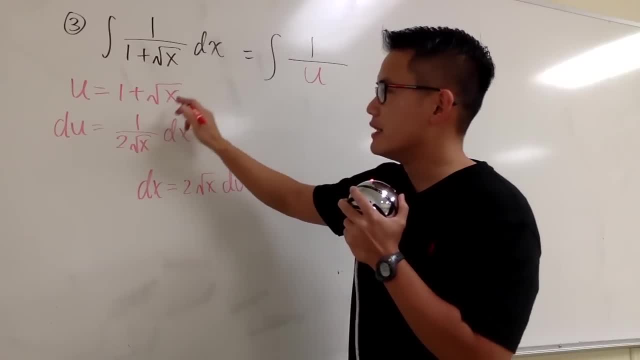 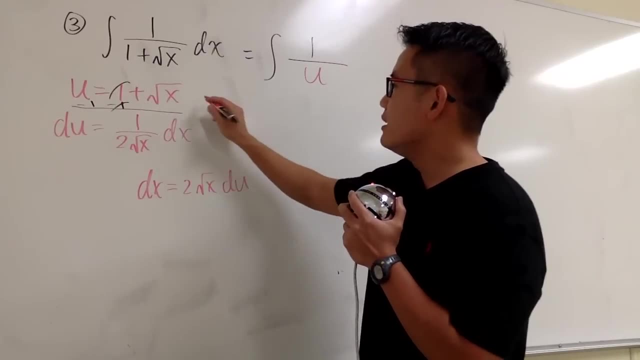 you see, u is equal to 1 plus square root of x. Why don't we just subtract 1 on both sides? This way we get what. This way, we can see that square root of x is equal to u minus 1, right. 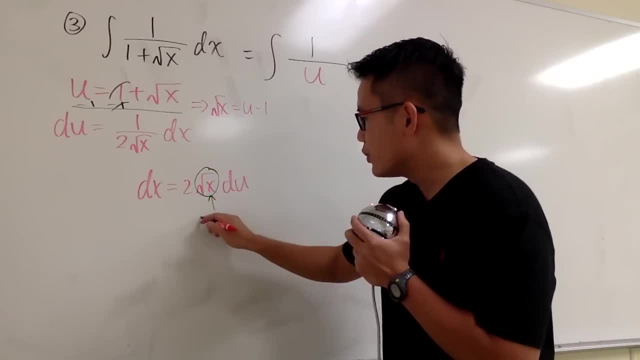 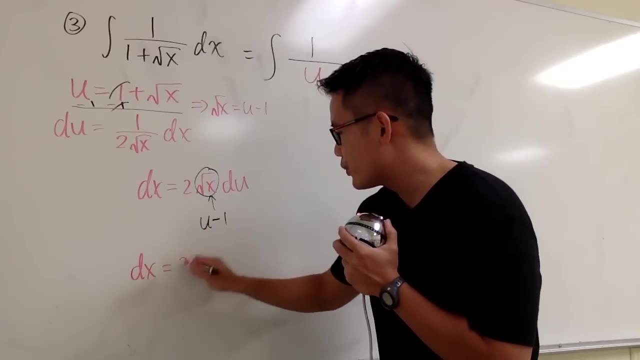 So you know this right here is the same as u, And we can rewrite this again for you guys. This is saying dx is equal to 2.. The square root of x is the u minus 1, so I have to use a parenthesis. 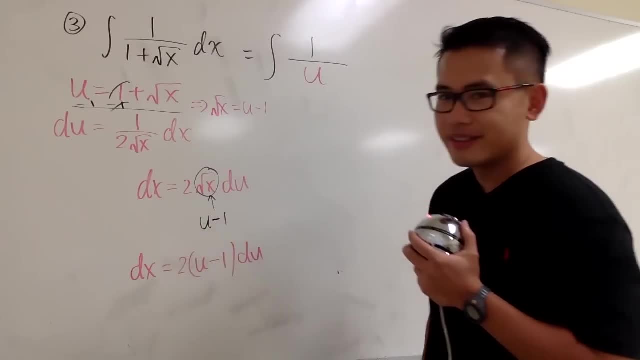 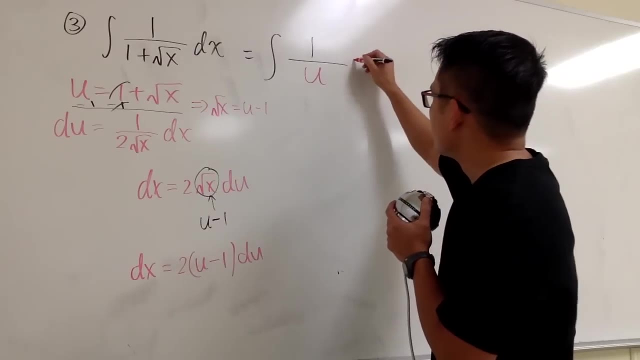 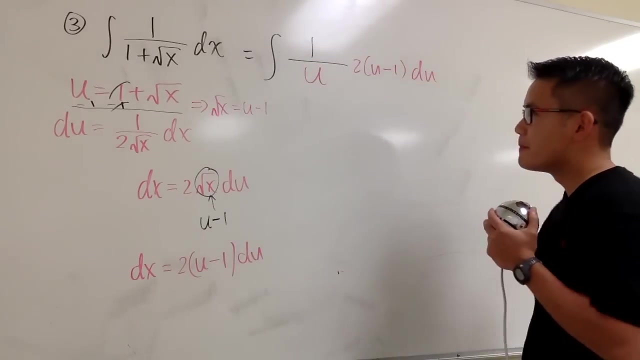 So we have the u minus 1 here and then du, And if I plug in this into the dx, that's what will happen, right? So let's write down 2, parenthesis- u minus 1, du, Okay, Okay. 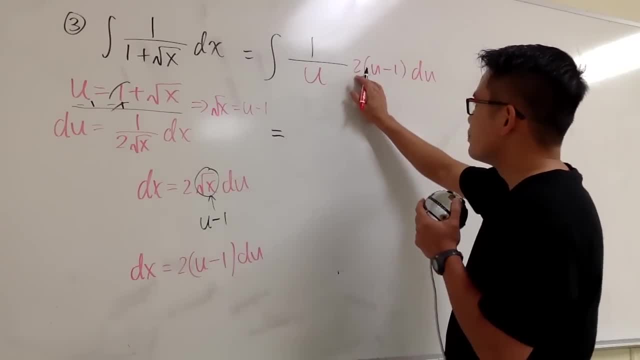 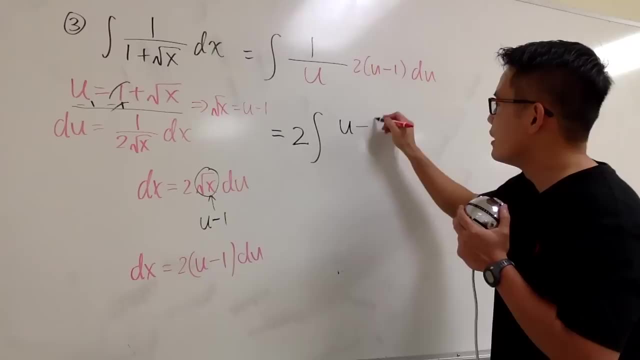 And now let's continue. A few things that we can do. First, let's bring the 2 to the front, And then we have the integral u minus 1 goes on the top right Over u, And this is du. 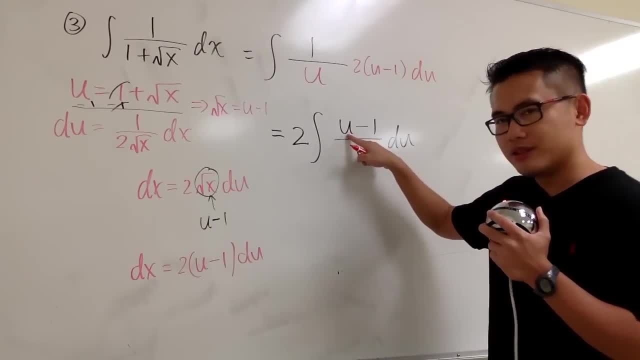 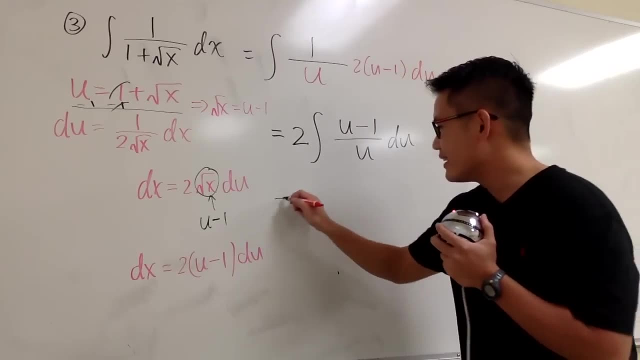 And now what? Well, I cannot just integrate this u because this u is affected by this u, So we are going to split the fraction. Okay, This is going to be 2 integral u over u. Let me write down all the work for you guys. 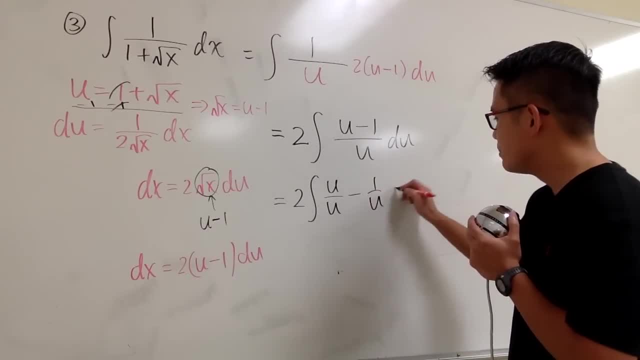 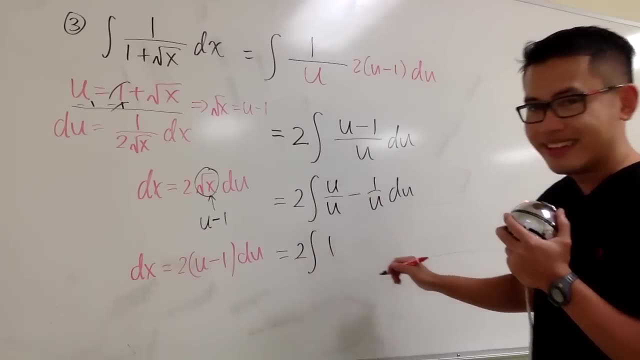 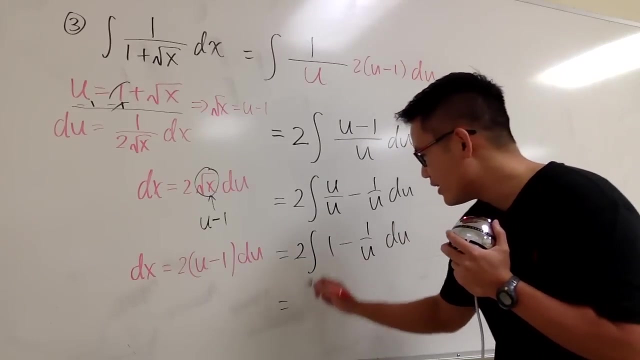 And then minus 1 over u. We split the fraction And we know this is just 2. integral u over u is 1.. And then we have the minus 1 over u, du And we're ready to integrate. So this is going to give us 2.. 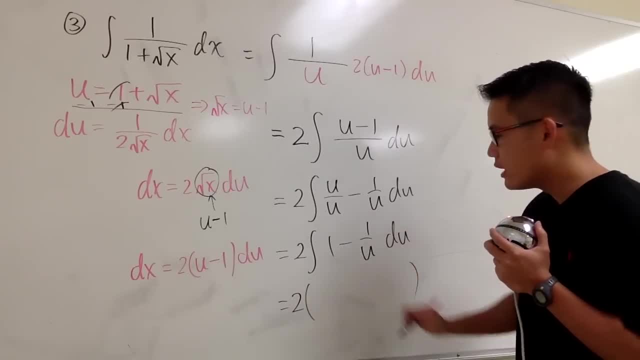 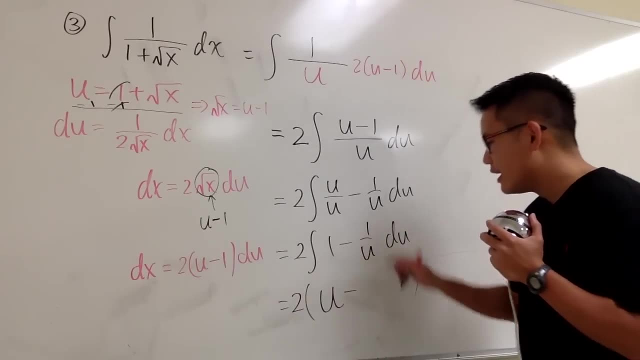 And let's open a parenthesis: for the resolved integration, 1 in the? u world, the integral for that is going to give us u And then minus The integral of 1 over u in the? u world, that's ln absolute value of u. 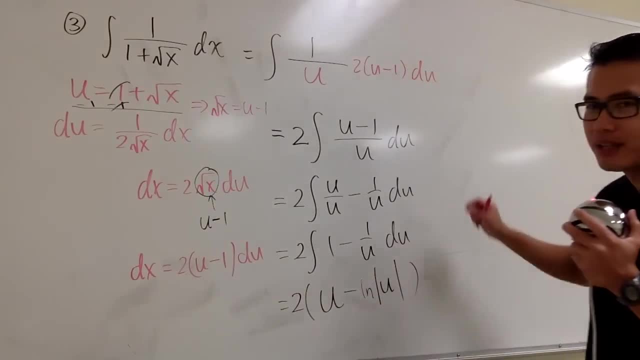 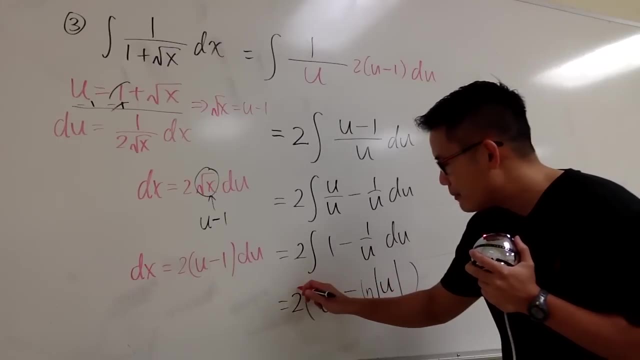 And then we are done. And now I have to take this back to the x world. We were done with the integration part right? So I'm going to do two steps right here. I'm going to take the 2 and the distributing side. 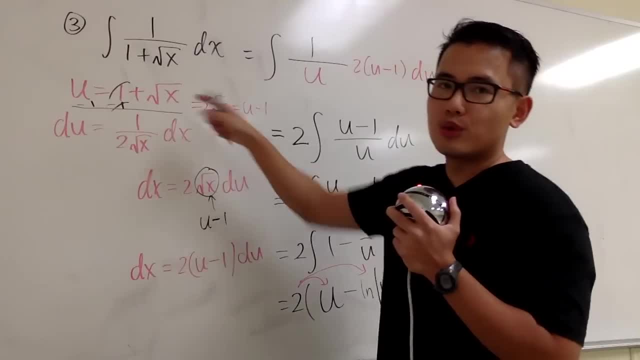 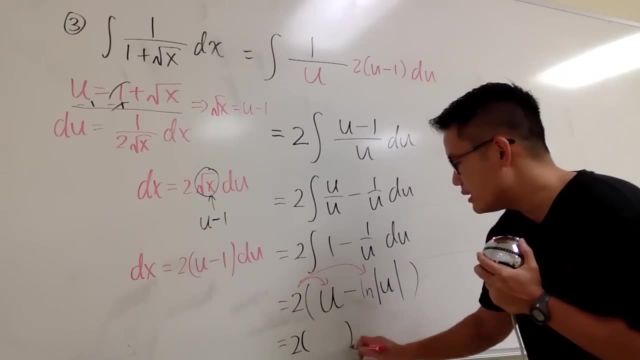 In the meantime, we know u is equal to 1 plus square root of x. right, That's what we said to start off with. Therefore, we will have 2 times the parenthesis. So the parenthesis u is 1 plus square root of x. 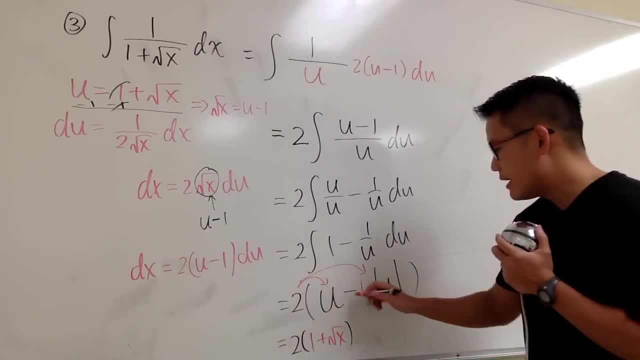 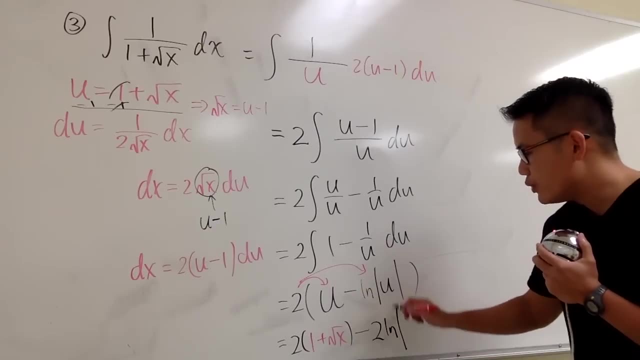 So let's write it down right here. And then minus 2 times that, So we have 2 right here. And then ln absolute value: The u is 1 plus square root of x. So let's put that down right here. 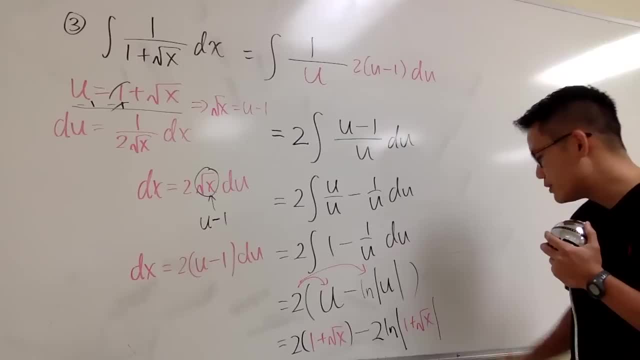 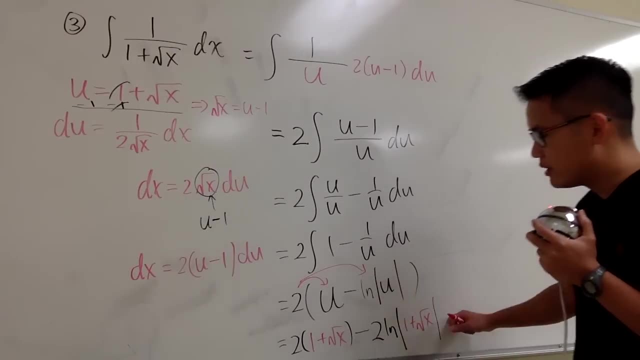 1 plus square root of x And we close this absolute value And technically we are all done right here. But a few things I'm going to mention in this particular video. But a few things I'm going to mention in this particular video. 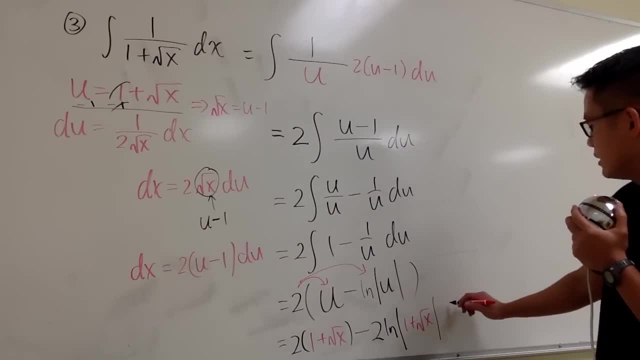 But a few things I'm going to mention in this particular video. First, as you can see. First, as you can see. of course we can distribute a 2 in this parenthesis right. of course we can distribute a 2 in this parenthesis right. 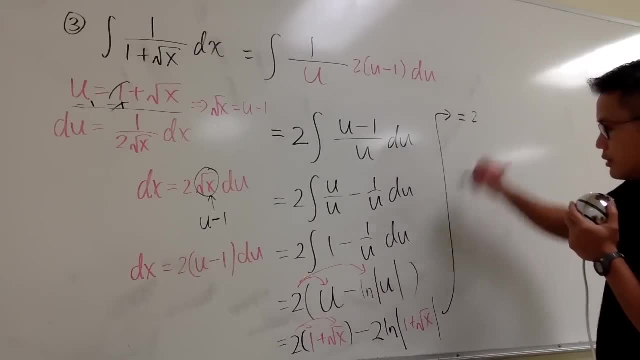 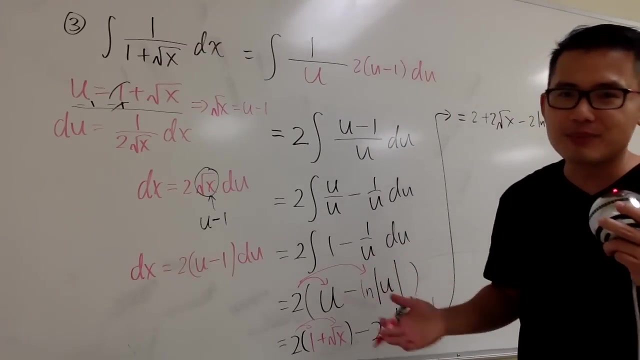 in front of this parenthesis And we'll end up with like all this, isn't it Alright and the moment we are done? Alright, and the moment we are done be plus c. but you may find the answer to be different in the back of the textbook, if you have. 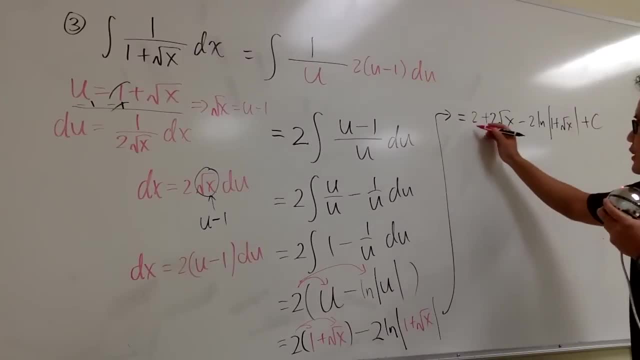 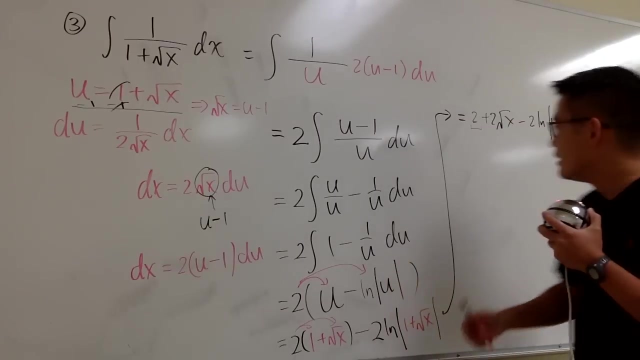 this question for the homework. first, you see, you have a constant right here, which is the two, and then when you have two plus c, this is a constant. this is also a constant. two constants. when you add them together it is still a constant. so sometimes they may merge into just one big. 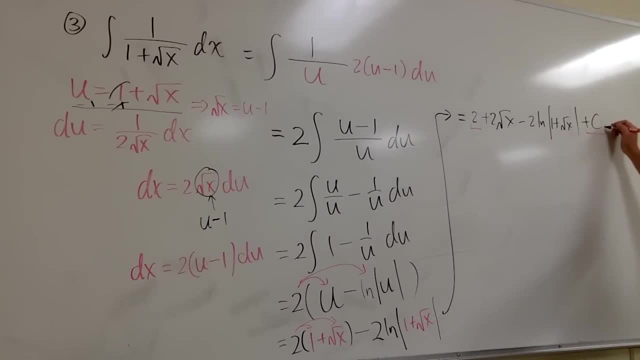 constant c. so right here, i would like to label this as c1, and what you can do is you can ignore the two, but then just kind of label this as a new c. just write on the function part, that's all. so let's write down two and then we have the square. 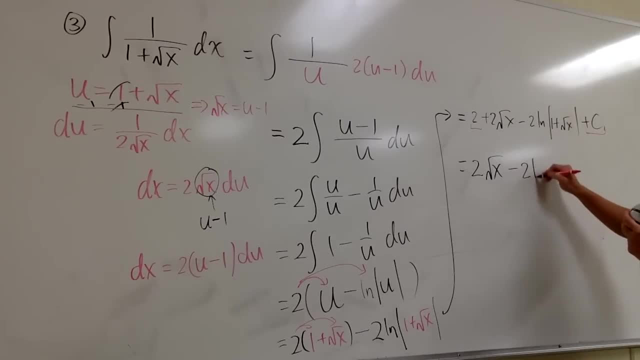 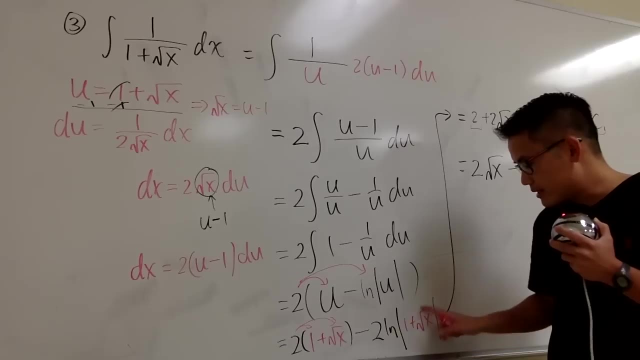 root of x minus 2, and then we have the ln. and now- this is another thing i want to mention. if you look at this part right here, we know square root of x, the output is always what the output. So the output of square root of x is always positive. and then we are adding, and this is the positive one. 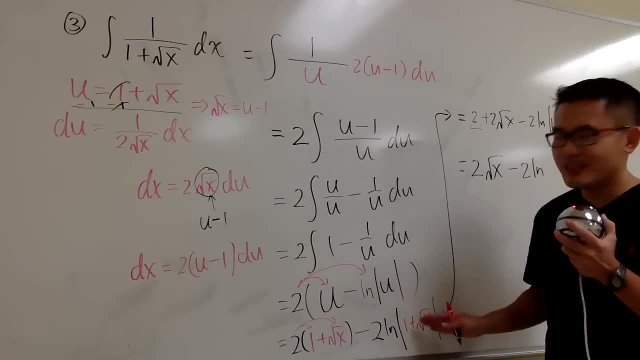 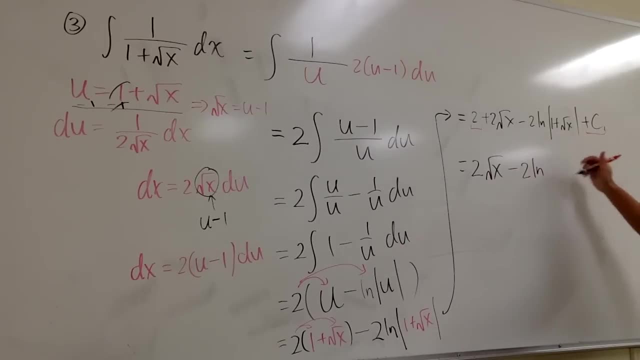 Positive plus a positive inside. here we are always guaranteed to have something positive. In that case, the absolute value is not needed. Therefore, I can change the absolute value into just a regular parentheses and then put in 1 plus square root of x. 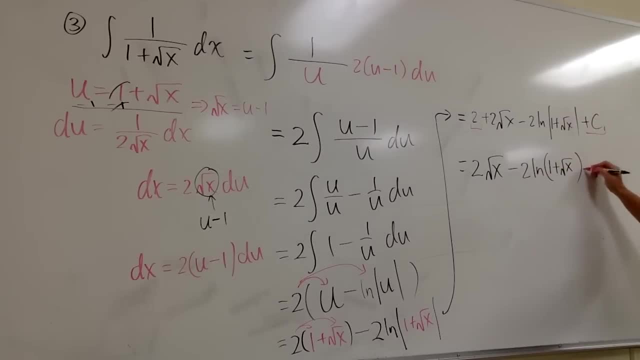 And, as I said this and that together, I'm just going to write it as another constant, so plus c, and technically I will label that as c2.. However, this is what I'm going to present for the answer. In that case, I will just write this as the constant that we are going to use and this, right here is it. 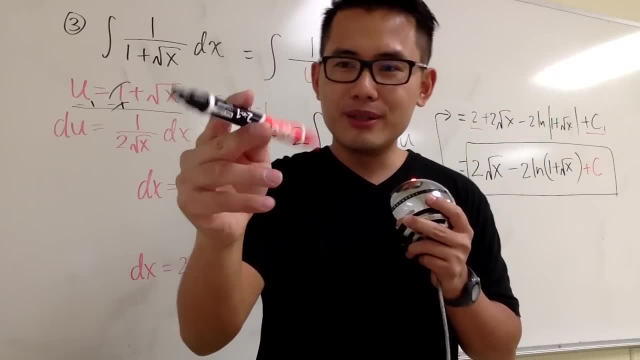 That's it. Let me know what you guys think about this black-red marker. It's really cool, isn't it?